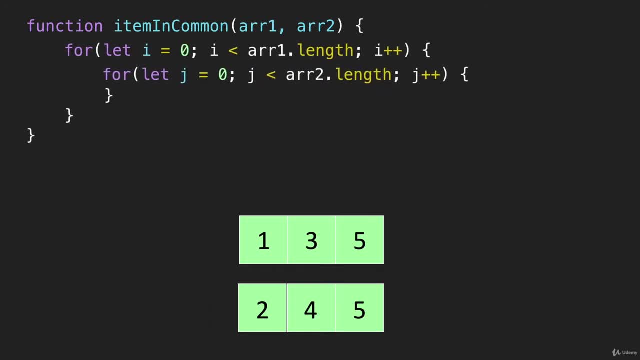 through the first array, a nested for loop that goes through the second array, And if, at any time, these match, we'll return true. Otherwise, if we go through these for loops and don't find any matches, we'll return false. So let's just flip over to Chrome DevTools and take a look at this. 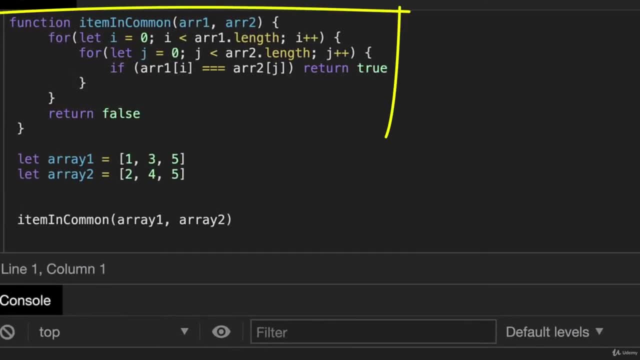 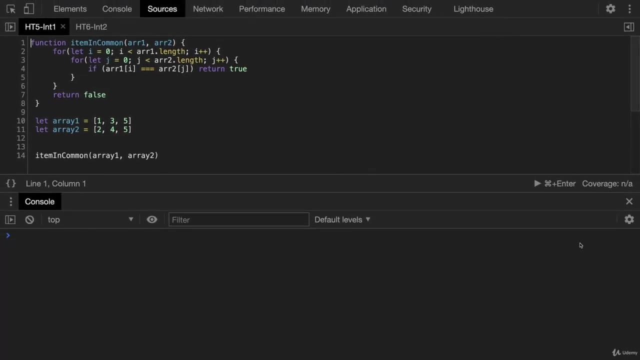 So there is the function we just wrote. These are the two arrays and we will run the function here. So when I run this we'll either get true or false. And we'd expect true because we have those two fives that are items in common. So I'll run this And sure enough, that is true. And then on array: 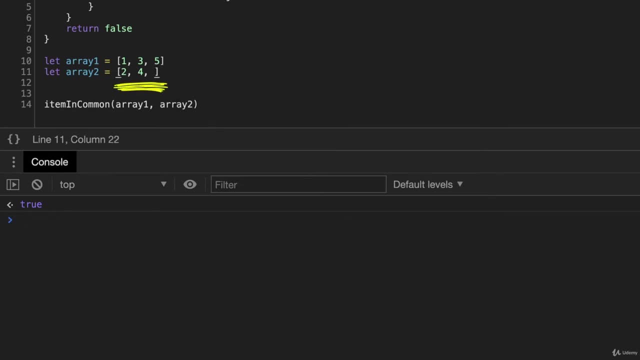 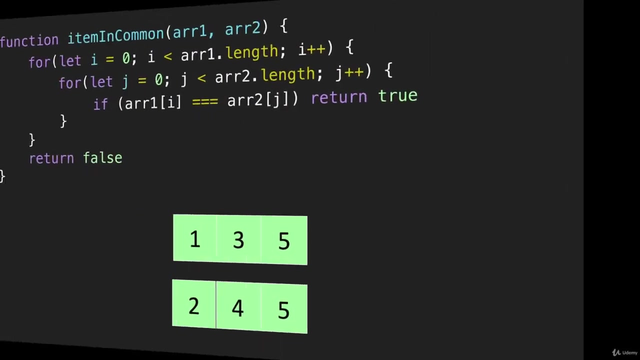 two. I'm going to change that five to a six, And then I'll run this again And we get false. So this works, It's just not super efficient, Okay, so now let's flip back. So this is where we left off here, But there's a more efficient way to. 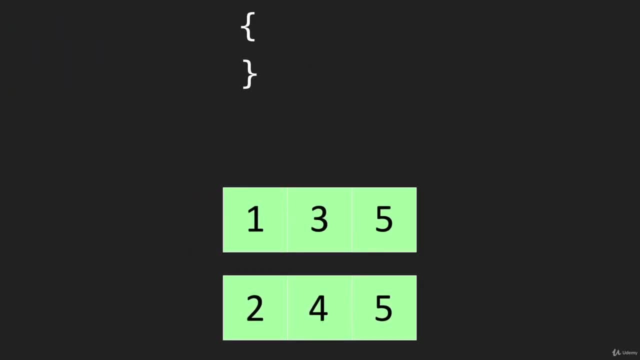 do that, And that is with an object. So this is what we're going to do: We're going to loop through that first for loop, And each of these numbers one, we will add this, the object, that's the key. And then we're going to add this to the object, And that's the key, And that's the key. 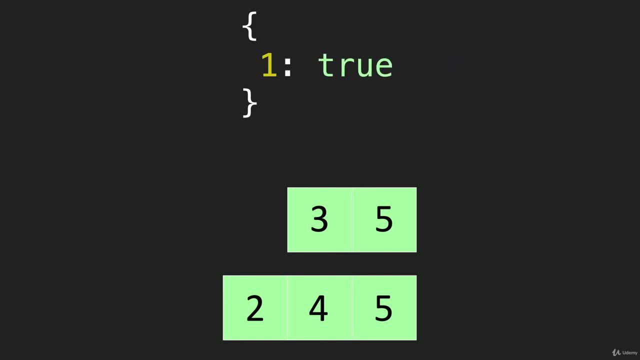 With a value of true And we'll do that for the next item in the array, Set that to true and the next item in the array, And we'll set that to true. So now what we can do is just loop through the second array and say: is two in this object as a key, And that is an O of one operation, And then 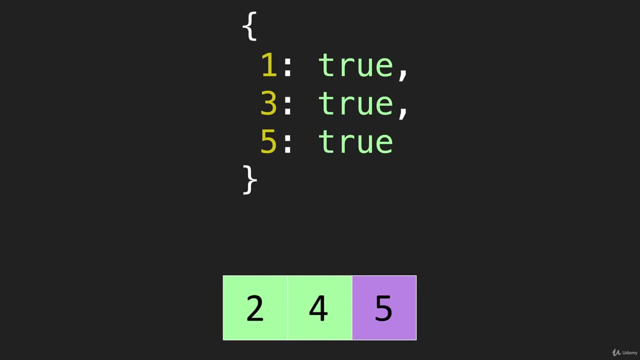 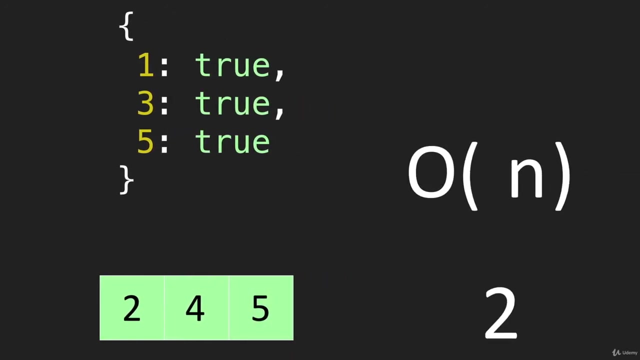 we can check the number four and then check the number five and it's finally going to come back. true, But the difference here is that the number of operations is far less. we went through each array one time only, So you could say that that's O of two n, But of course we drop constants.